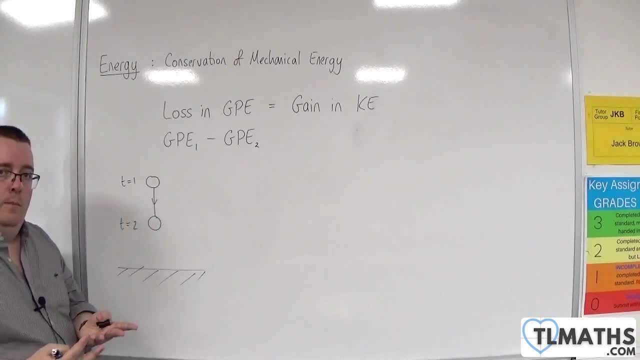 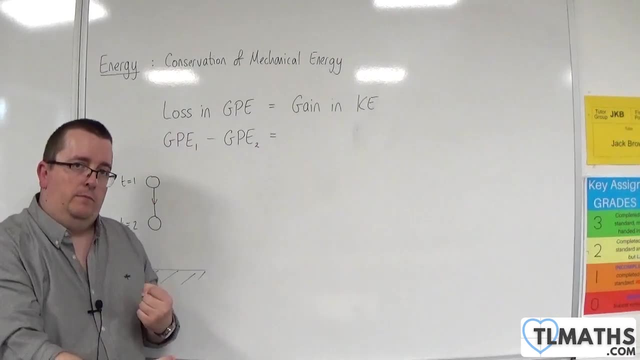 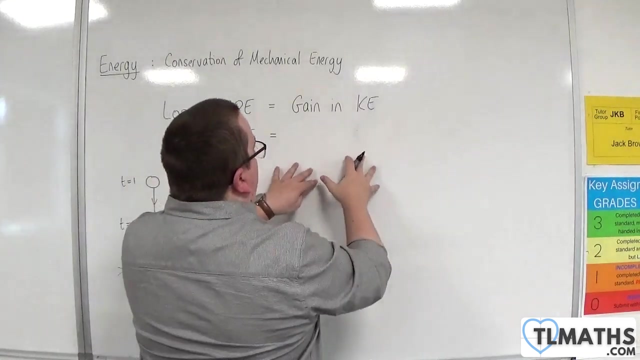 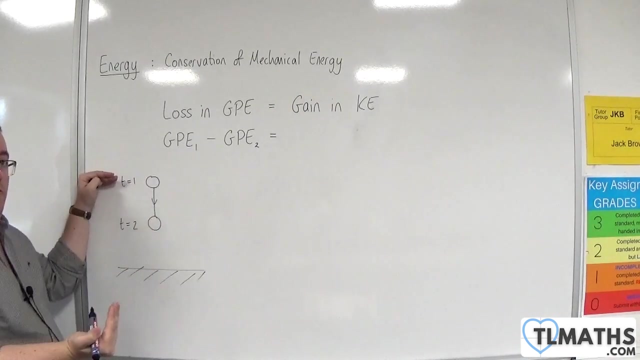 So as it falls, it loses potential energy, gravitational potential energy. That energy must be converted into something, okay. So if energy is lost, it must be gained elsewhere. This is the idea: Conservation of mechanical energy. Now the gain in kinetic energy. well, initially the kinetic energy is zero. if we drop it from rest, okay. 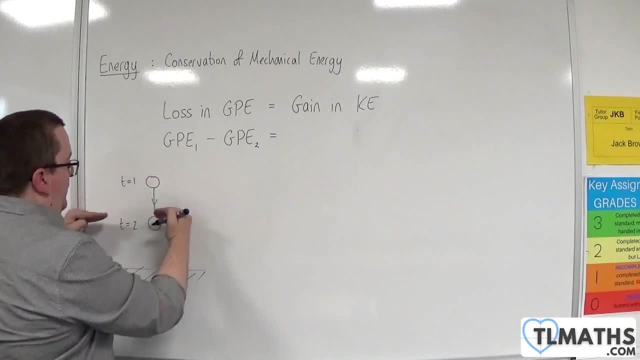 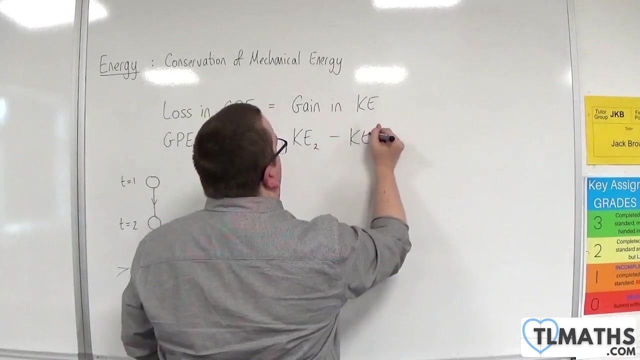 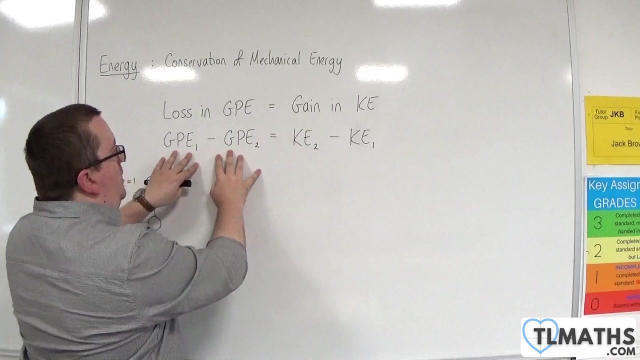 There's nothing. But by the time it gets here it will be travelling faster and so it will have more kinetic energy. So we can write the kinetic energy at time two, take away The kinetic energy at time one, So this is the loss in gravitational potential energy. 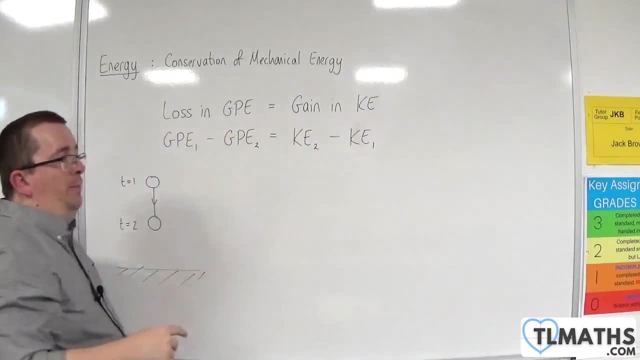 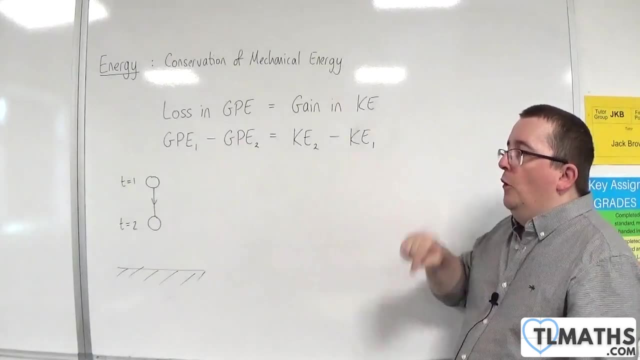 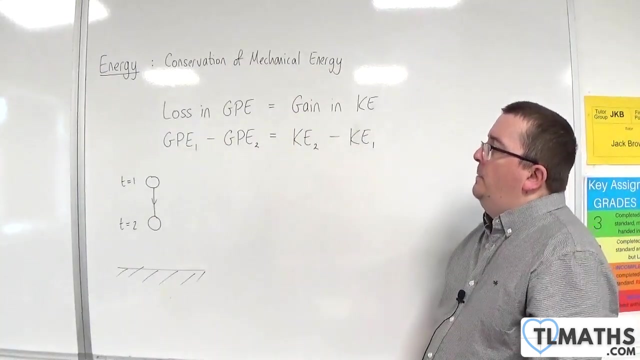 This is the gain in kinetic energy And they must be the same. if the force due to gravity, so the weight, is the only force which does work on the body on the ball, that's falling okay. So you need to think about this idea with energy. 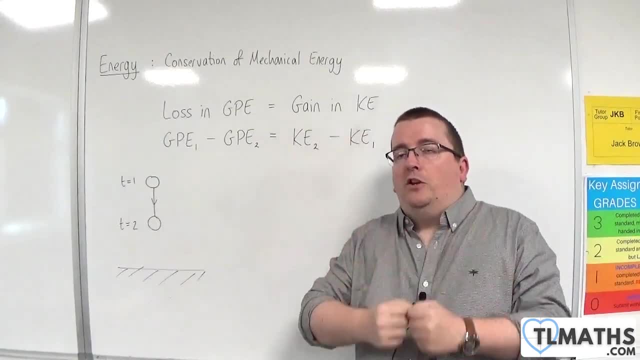 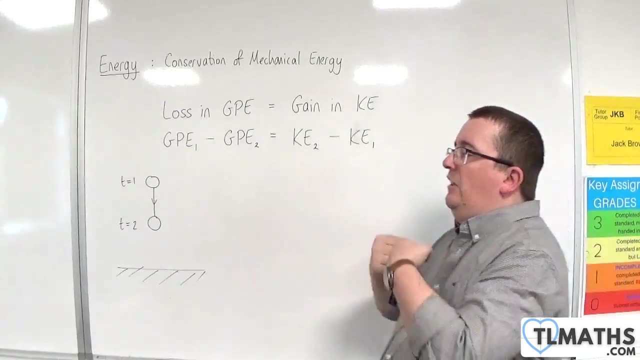 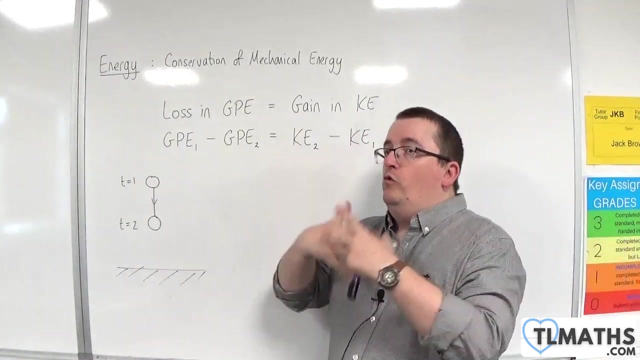 You need to think about this idea of it's being converted from one form into another. okay, So the gravitational potential energy in this case, is being converted into kinetic energy. Now, in reality, of course, you would also have to account for things like air resistance, things like that. 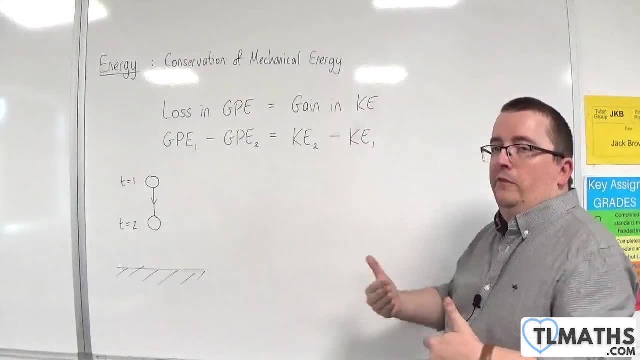 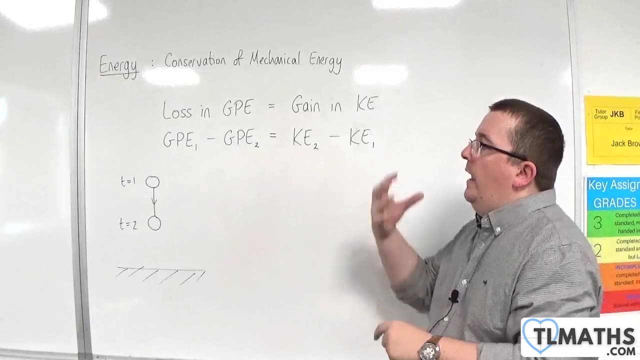 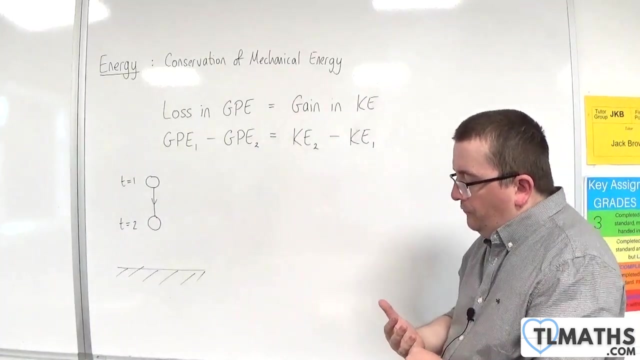 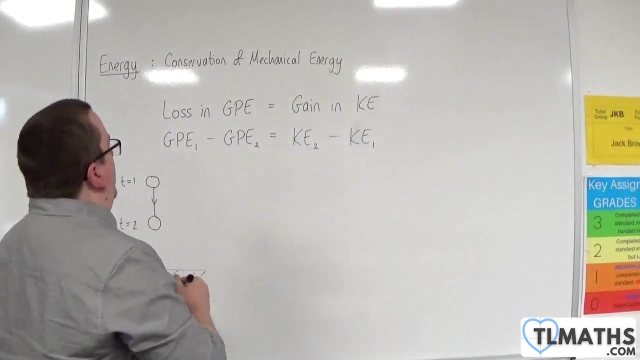 We'll talk more about dissipative forces in a bit, But this is the conservation of mechanical energy. if the weight is the only force acting on the body, okay, Now this can be rearranged into a neater form thinking about, if we just think about time one on one side and time two on the other. 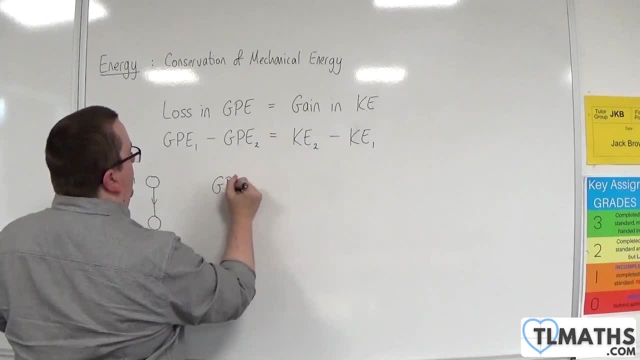 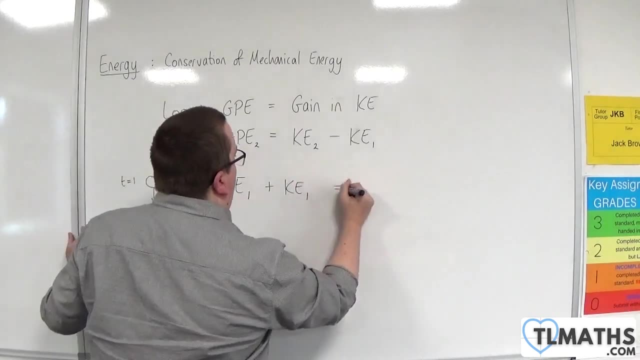 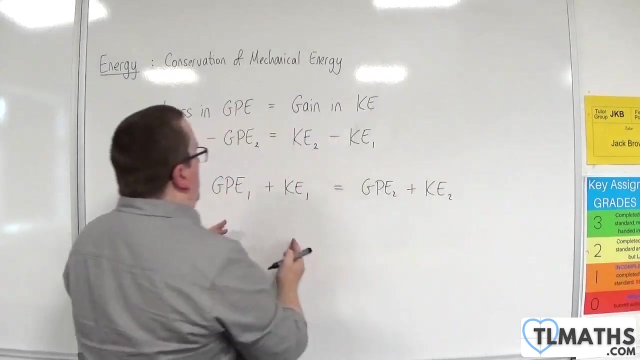 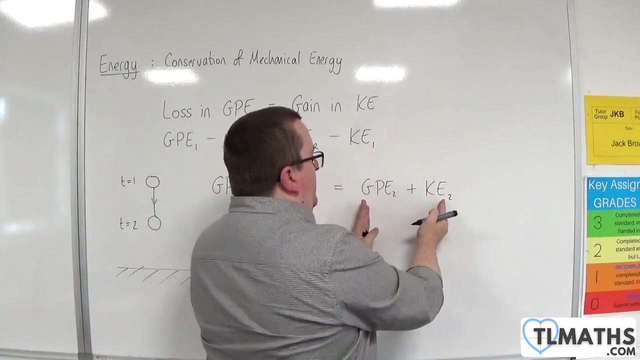 So you could write this as gravitational potential energy. So we got the gravitational potential energy 1 plus the kinetic energy. 1 is equal to the gravitational potential energy 2 plus the kinetic energy 2.. So the initial gravitational potential energy and kinetic energy must be equal to the final gravitational potential energy and kinetic energy.